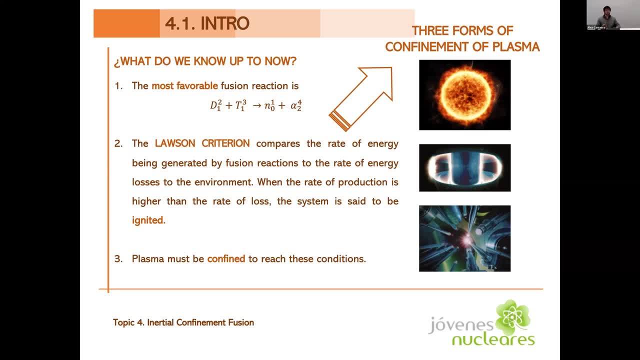 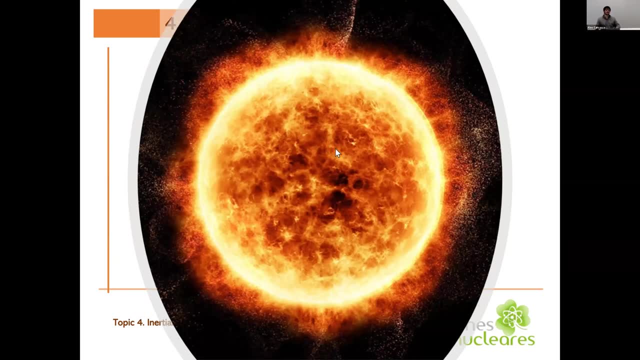 And we have three ways of doing this. The first way- and don't be scared- is whoa is gravitational confinement. This is the one that happens in the Sun. So, in the Sun, the light that we have outside is happens because the force of the Sun, of the Sun's gravity, confines the particles of and produces fusion, creating this, this light energy. 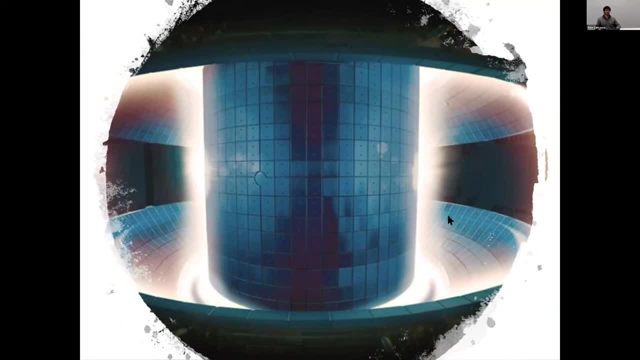 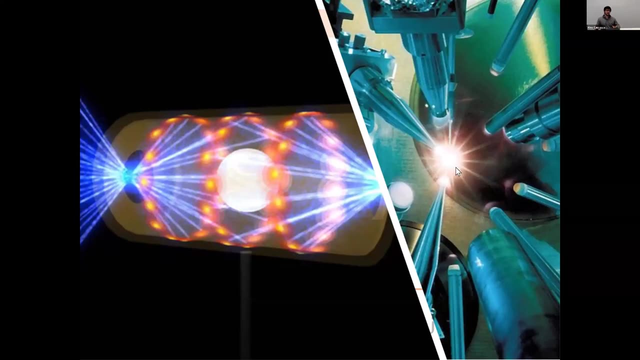 The second way is what Enrique presented before: magnetic confinement fusion: where a plasma is, is confined by a magnetic field. And the third way of confinement that we, that we know of and that we use is inertial confinement fusion, which is the one with all where, with all the lasers. 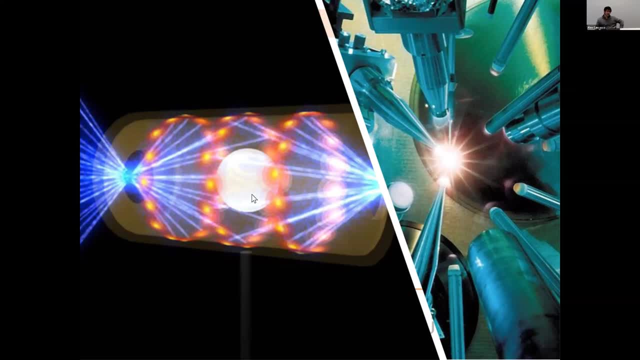 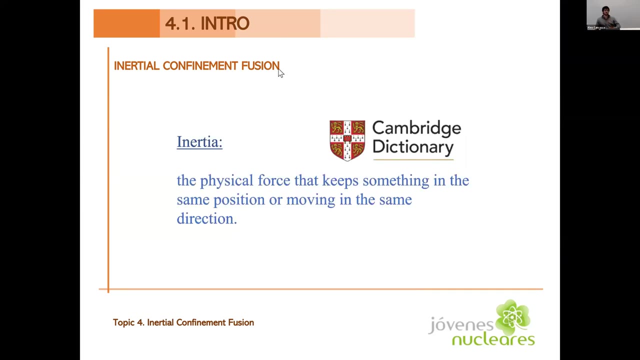 We have lasers that shine on a small capsule and compress the capsule, creating a fusion in the fuel that is inside the the capsule. So, as part of the- the last part of the introduction, this is called inertial confinement fusion, So inertia. Inertia is defined by the Cambridge Dictionary. 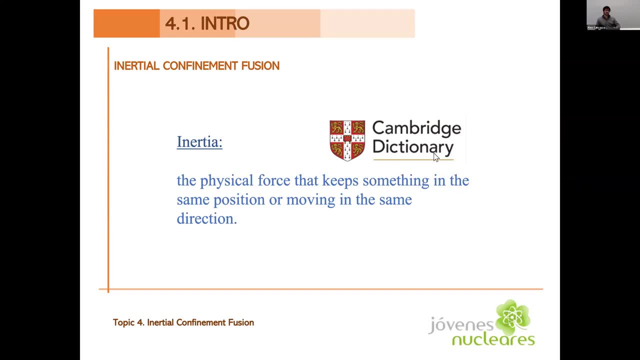 as the physical force that keeps something in the same position or moving in the same direction. So if something starts moving in a direction and it has enough acceleration, it will continue moving in that direction and this is caused by inertia. So we're going to use this force to to confine our plasma in this kind of in this kind of fusion. 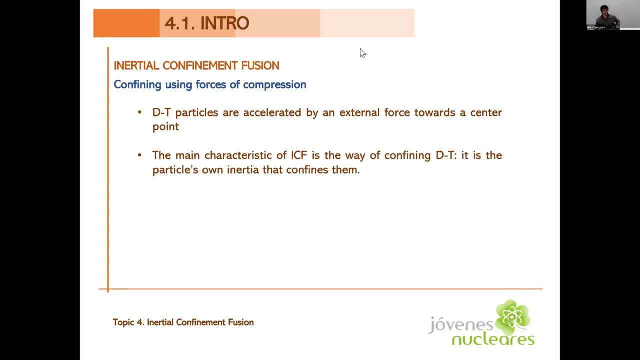 Deuterium and tritium particles are accelerated by an external force towards the center point, the force being the laser, as we will. we will discuss later. And the main characteristic of ICF is the way of confining the deuterium and tritium. 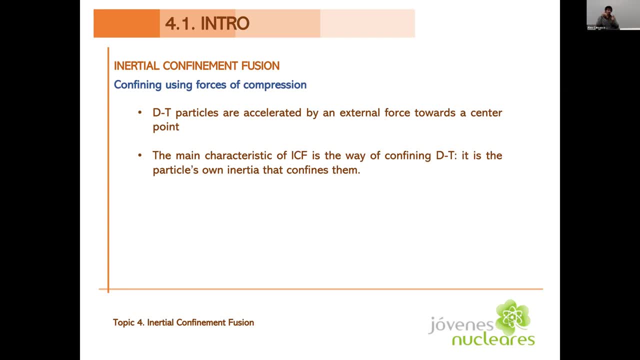 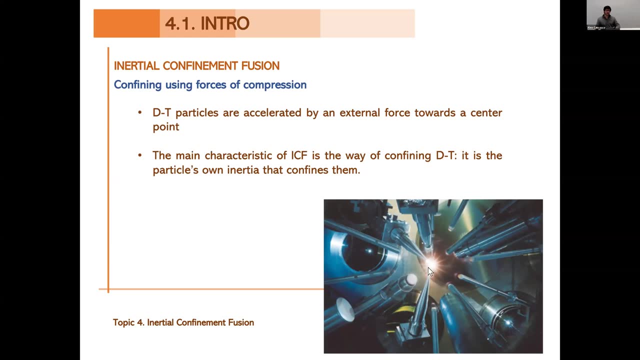 It is the particle's own inertia that confines it. Its own inertia towards the central point confines the, the plasma. So the lasers are shown on the particle, compressing it and compressing the deuterium and tritium in its interior. 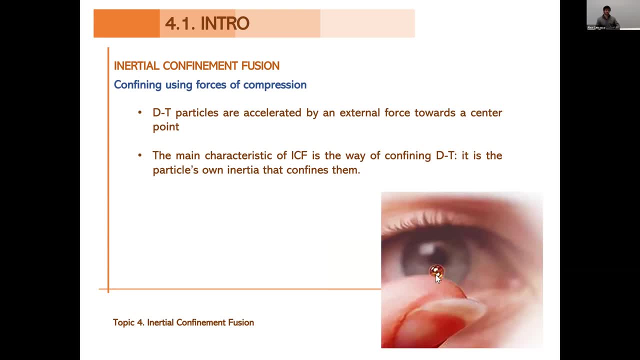 The particle is very, very small, as we see in this picture, only about 2 millimeters in diameter, and the, the fuel, would go inside the, the, the, the capsule. And when we compress the, the capsule, as we will see later, the fusion is obtained in the in the center. 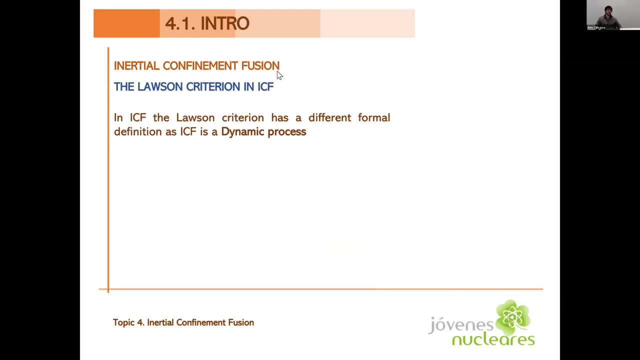 So for the last part of the introduction, as Enrique discussed the Lawson criteria in in magnetic confinement fusion, we will discuss it in inertial confinement fusion. The main difference is that it has a different formal, a different formal definition, because this is a dynamic process. 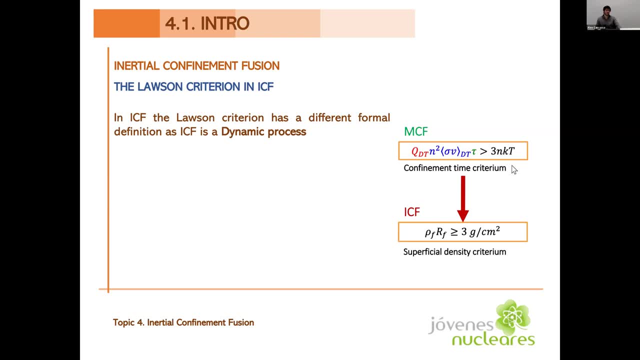 What does this mean? That in magnetic confinement fusion there's a time criterion to to fulfill, and in inertial confinement fusion the criterion is of superficial density. So we have to obtain a certain density in a certain area to confine the plasma. 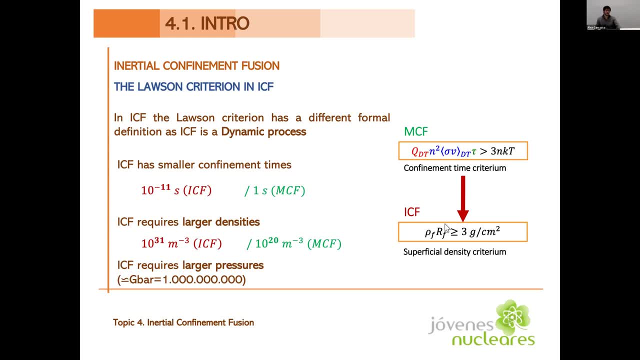 This is the. this is the way in which the Lawson criterion would be expressed in inertial confinement fusion. So this results in the fact that inertial confinement fusion has smaller confinement times than magnetic confinement fusion. It requires larger densities and it also requires larger pressures- up to one bigger bar. 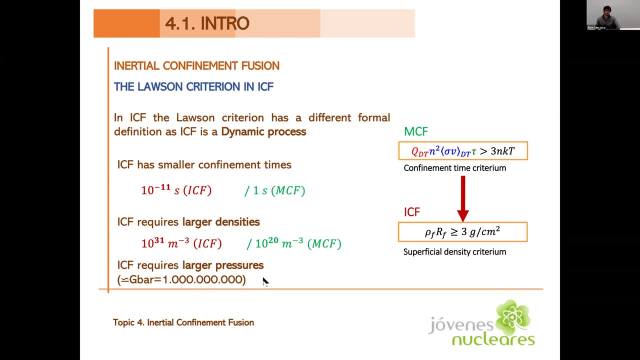 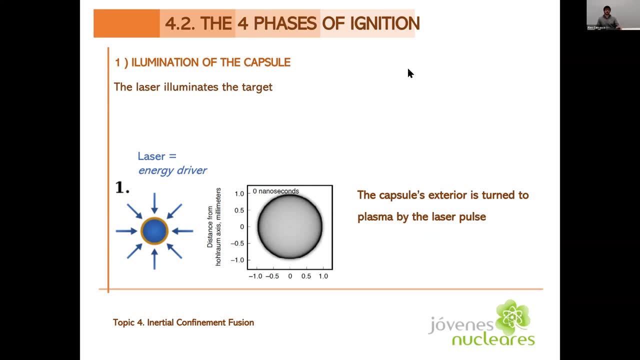 which is 1,000 million times the atmospheric pressure. So now we're going to go into the second part of the presentation, the four phases of ignition. When the laser shines on the, on the capsule, how, How do we get fusion? 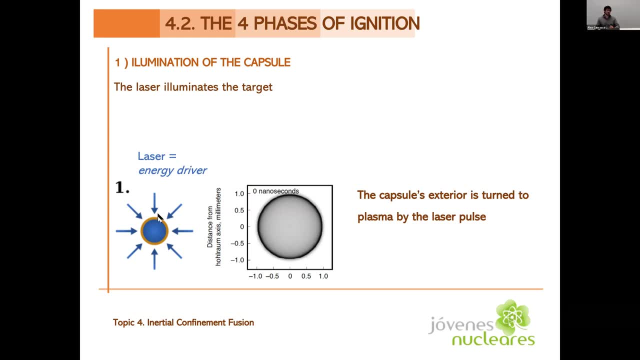 Firstly, the laser illuminates the target, the target being the capsule, and we're going to call the laser the energy driver, because it's what gives us, gives us energy for the reaction. It illuminates the target, compressing the capsule. 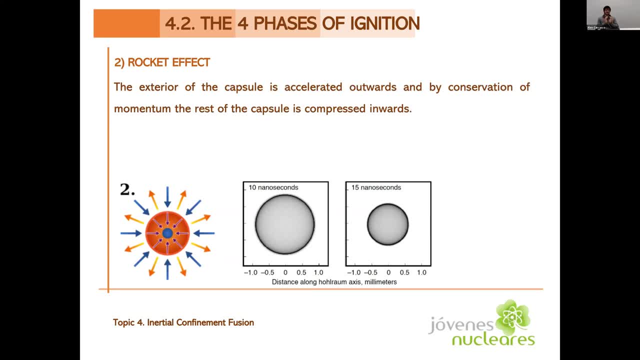 and making the exterior of the capsule accelerated upwards. If the exterior of the capsule turns into plasma because of the high, high, very high altitude energy deposition by the laser and shoots outwards, this pushes the interior of the capsule with the fuel inwards, compressing it. 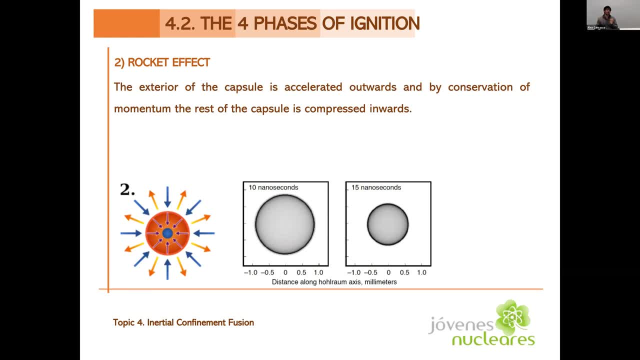 This is called the conservation of momentum, or or or action-reaction. you know, And it's the same, it's also called the rocket effect. Why? Because in a rocket, when a rocket shoots upwards, it shoots upwards because it's shooting gas downwards. 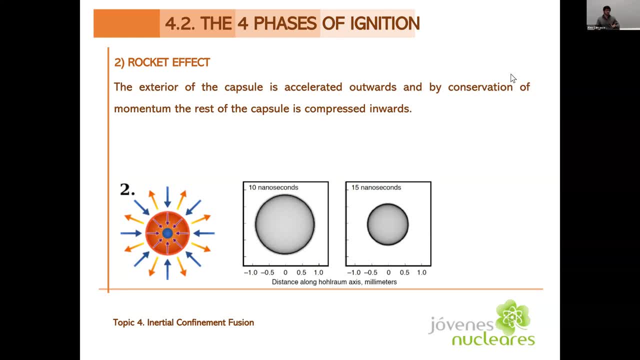 and the fact of pushing the, the gas downwards, pushes the rocket up upwards by, also by conservation of the, of the linear momentum. no, And this is the same effect that we will apply in fusion. So we shine the laser, the exterior shoots outwards. 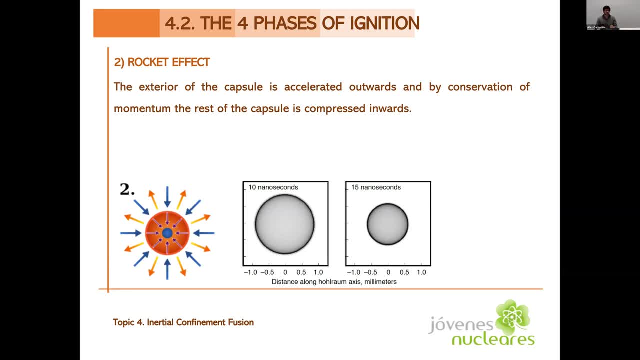 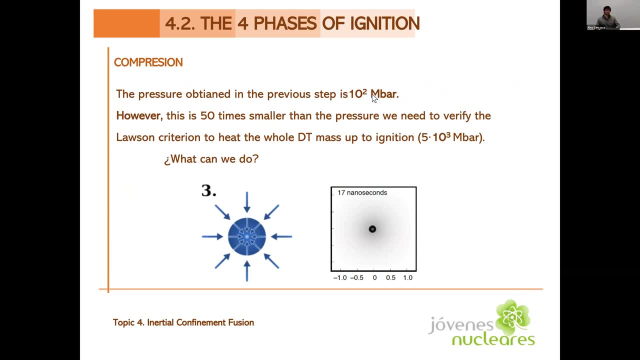 and the interior compresses the fuel compresses. However, what is the problem? That with our, with the lasers that we have nowadays, we can only obtain in this way a pressure of 10 to the 2 megabars. This pressure is 50 times less. 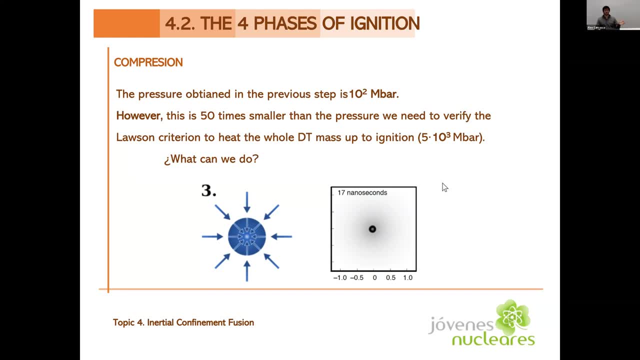 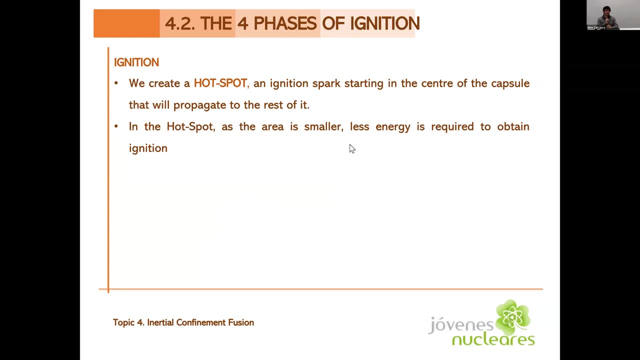 than what we said we needed in the Lawson criterion. So we have a problem here. What can we do? Well, the solution is to create a hotspot in the center of the of the of the fuel capsule. This means that we try to get ignition only in a small 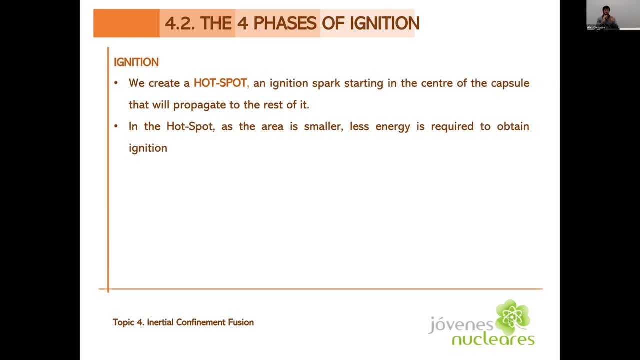 in the small, in the small center of the capsule and not in the whole capsule. at the same time, This is like a spark that starts in the center and propagates to the rest of the of the capsule. In this way, we need much less energy. 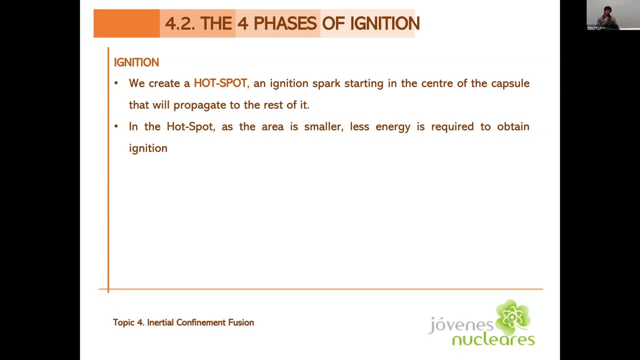 because the ignition happens only at a certain, at a very, very small place at the same time. So to recap, we have, first stage laser illumination. second stage, compression with the rocket effect, as we discussed. third stage, ignition in a central hotspot. 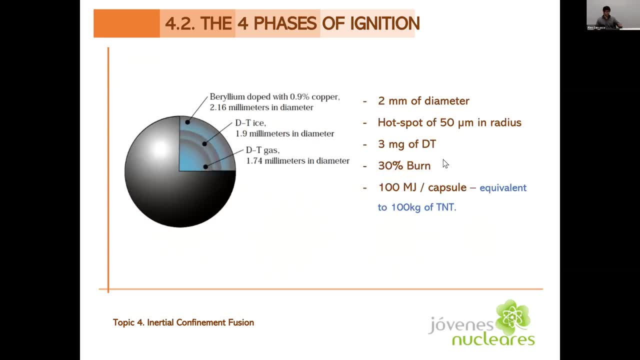 and fourth stage: burning of the capsule. So we have a capsule of 2 millimeters of diameter. we create a hotspot of 50 micrometers in radius. Inside the capsule we have 3 milligrams of deuterium tritium. 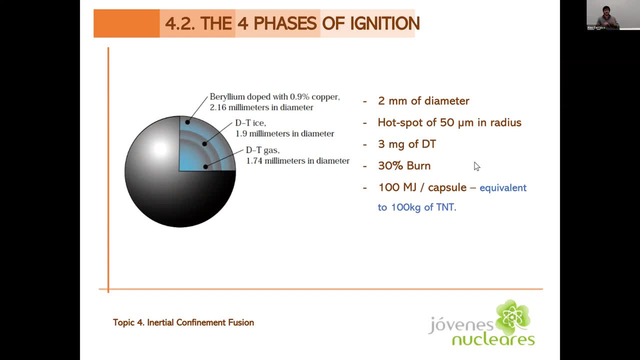 and we will burn 30% of this deuterium tritium. We can't get a burn of the whole, of the whole capsule, of the whole contents, And with this we produce 100 megajoules of energy per capsule. 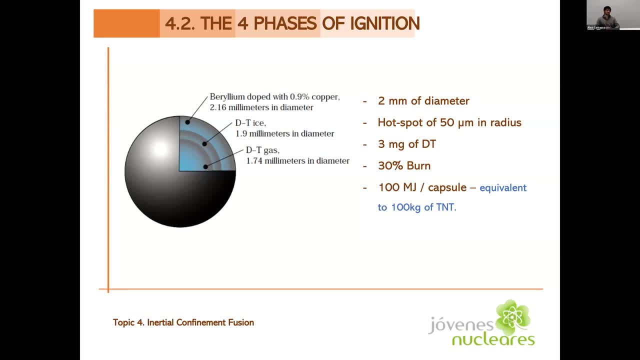 The problem with energy is that we oftentimes we don't have the, the orders of magnitude in our head for energy, because we're always talking in power, not the power of a nuclear power plant or the power of a produced by a by a. 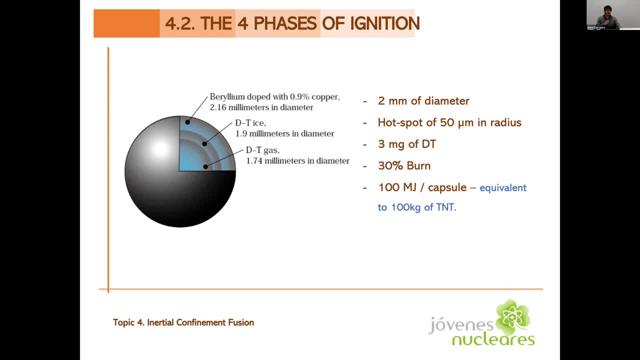 by a certain reaction or by a certain, by a certain fuel And in energy. the equivalent of 100 megajoules is 100 kilograms of TNT. So from burning 30% of 3 milligrams of deuterium tritium. 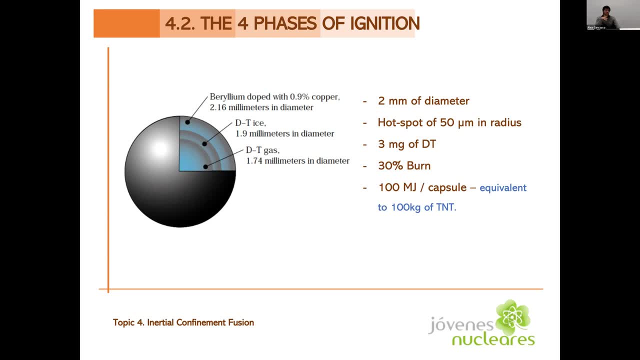 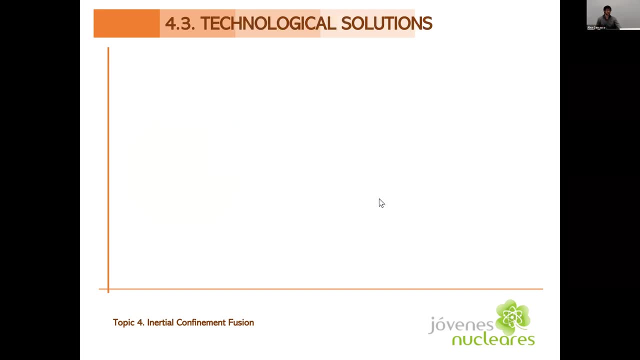 we're obtaining the equivalent energy to burning 100 kilograms of TNT, So it's fairly incredible. Now, after seeing the whole process of inertial confinement fusion, we're going to go through the technological solutions. How do we do we? 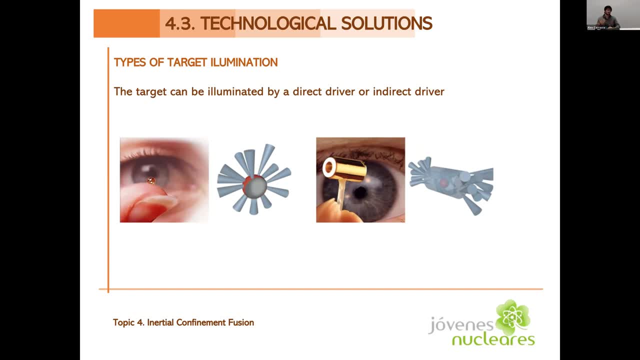 What are the technological solutions that we that we have, that we have found, to put this into into practice? First, we'll discuss types of targets of target illumination. The target can be illuminated by a direct drive or an indirect drive. 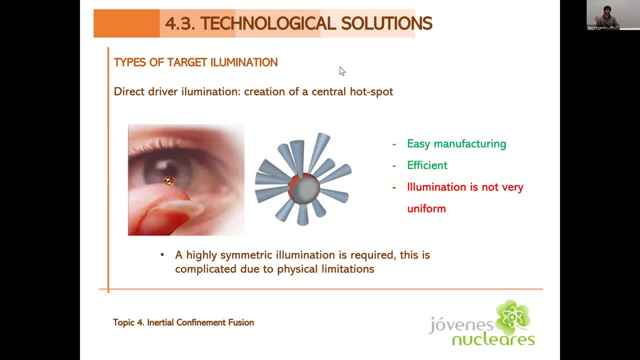 Direct driver illumination is the creation of a central hotspot. It is what we were discussing before. The laser shines directly on the capsule, compressing it and creating a hotspot in the center of the capsule. This has easy manufacture because we only have to create the capsule. 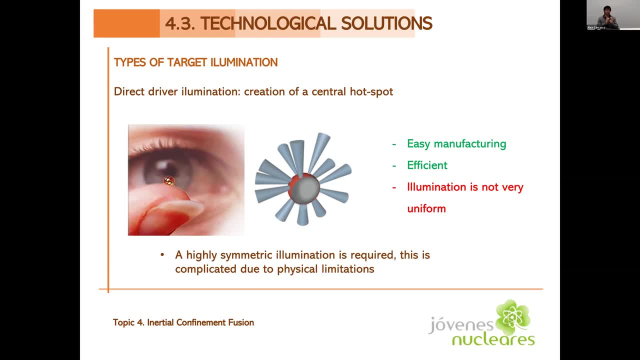 It is very fairly efficient because the laser shines directly on the capsule, And the problem with this is that illumination is not very uniform because the laser is very far away from the small capsule, So getting a uniform illumination is difficult. 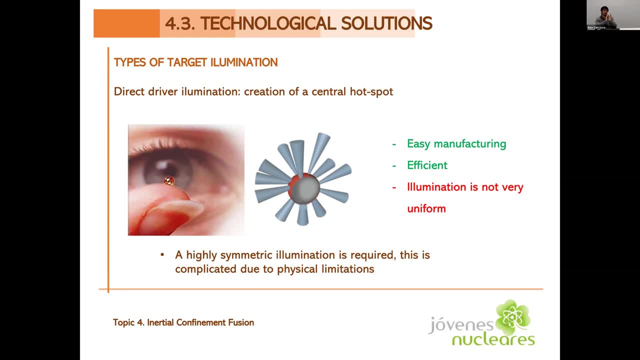 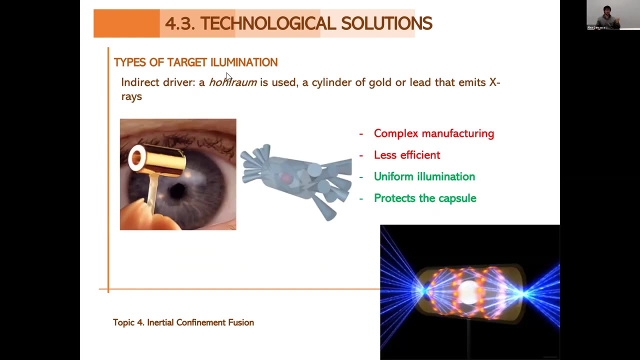 And sometimes we will end up with the capsule being compressed like a rugby, like a rugby ball shape, and the hotspot not being central. so the burn of the capsule isn't very, isn't very, very uniform. no, And with indirect drive, we, we resolve this problem. 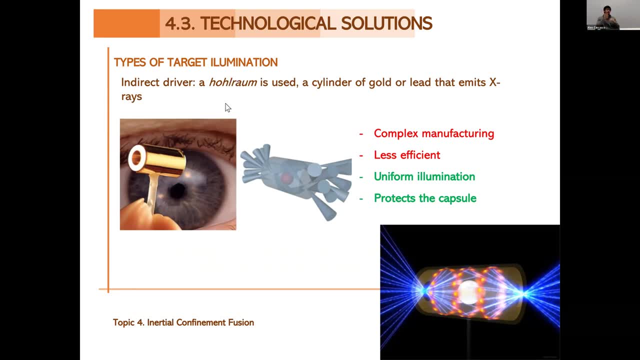 Indirect drive is when a laser shines on what we call a hochraum, and it is a cylinder of gold or lead, so a high, high Z number material that when the laser shines on the on the cylinder, this cylinder emits X-rays that then shine on the capsule. 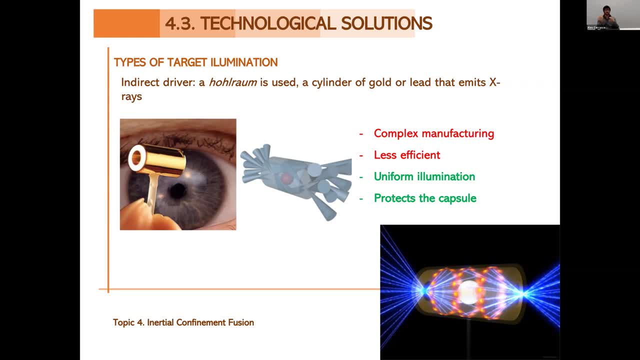 With this. what we try to to gain is a very uniform illumination of the capsule. As you can see in the in the picture in the bottom, in the bottom of the screen, the laser goes in, shines on the on the cylinder. 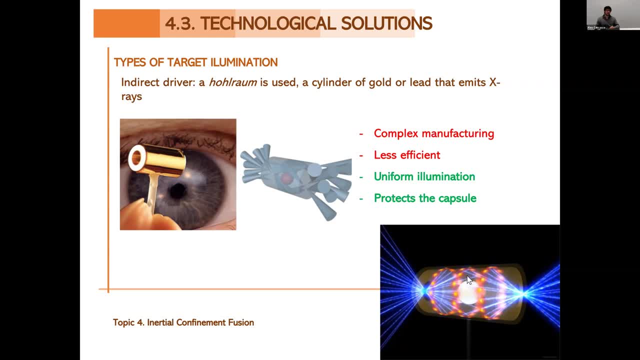 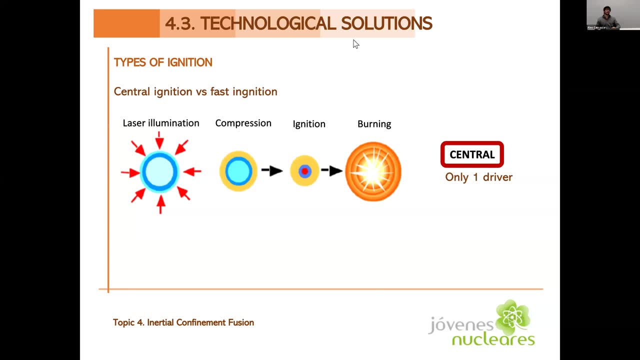 and the cylinder emits X-rays that shine on the capsule and produce produce fusion. The second: the second difference that we want to make in technological solutions is the types of ignition that we can have. We can also have two types of ignition. We can have central ignition, which is what we what we discussed before. 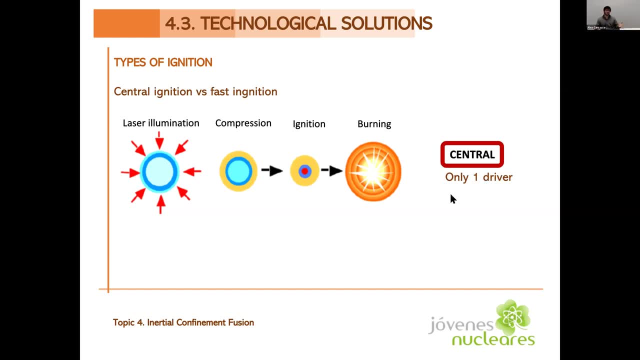 with only one driver. We only have one energy driver: the laser that shines on the on the capsule and produces the burn, the ignition and the burning. Or we can have fast ignition. where we have more than one driver, We will have a first: the laser that compresses the capsule in central ignition. 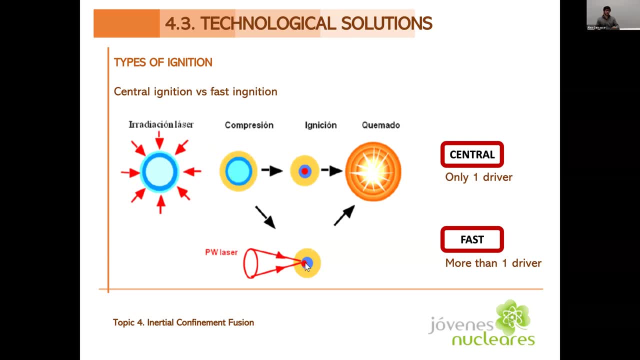 and then we will have a second laser that will start and will create the hotspot on in the, in the capsule, and it will and it will burn in this way, So you have a second laser. that's like the spark, the spark that creates ignition. 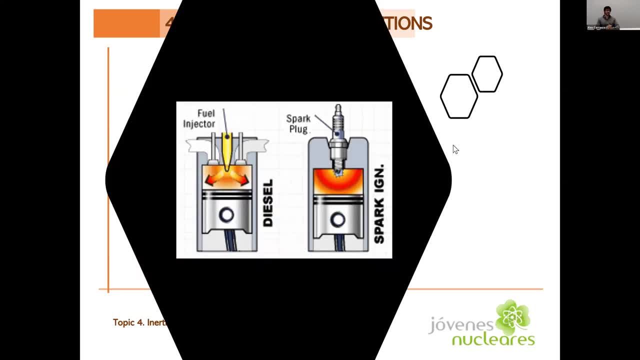 I really like to compare this, this to with a metaphor to to engines, to car engines. so if there are any engines engineers in the in the audience, they will. they will understand this meta with this metaphor, I think. 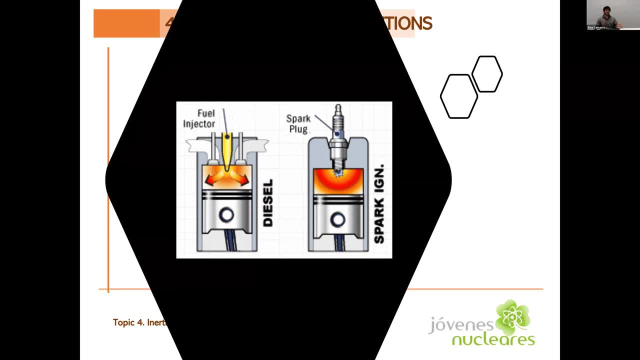 This is like comparing a diesel engine and a and a normal and a normal gasoline engine. The diesel engine compresses the fuel until it has ignition, and the gasoline engine compresses the fuel and then the spark plug produces a small spark that will then ignite the whole fuel. 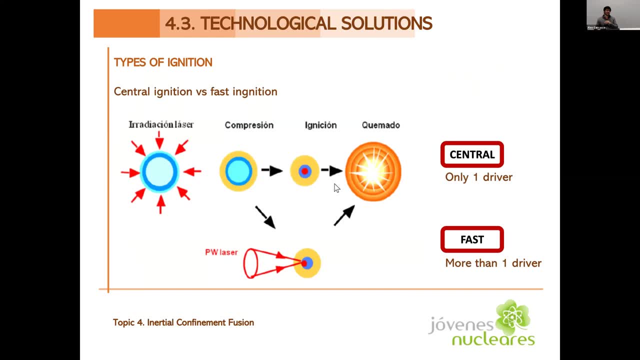 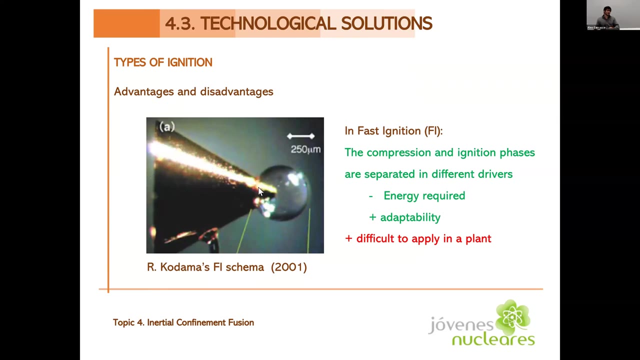 So, in the same way, central ignition would be like a diesel engine and fast ignition has a little spark plug in the form of another laser that produces the, the ignition. The concept of fast ignition that we see here is a is a gold cylinder. 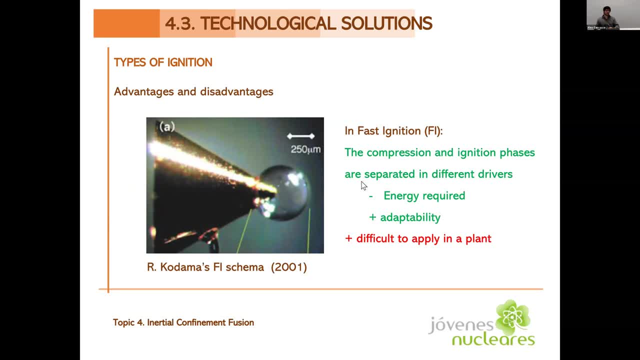 that protects the second laser that will enter the, the capsule producing fast ignition. So the the advantages of fast ignition is that the compression and ignition phases are separated in different drivers. This gives us. this means that we need less energy, and it gives us more adaptability. 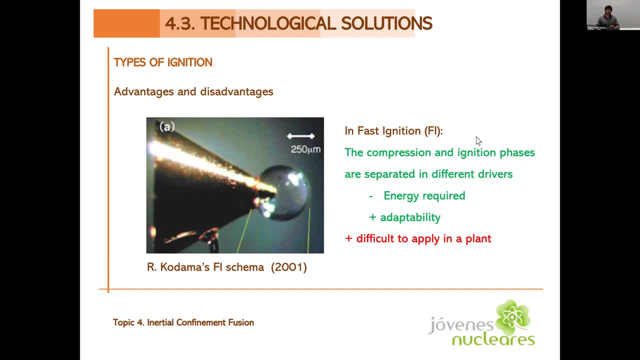 Because each laser can be can be can be more efficient for its own, for the each of the phases. One laser will compress, the other will ignite. So each laser pulse will be will be tailored to the needs of each of those phases. 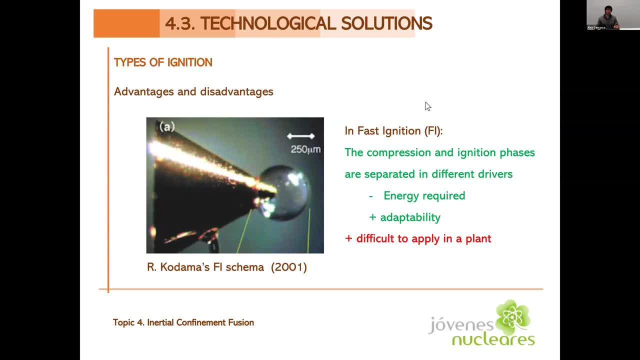 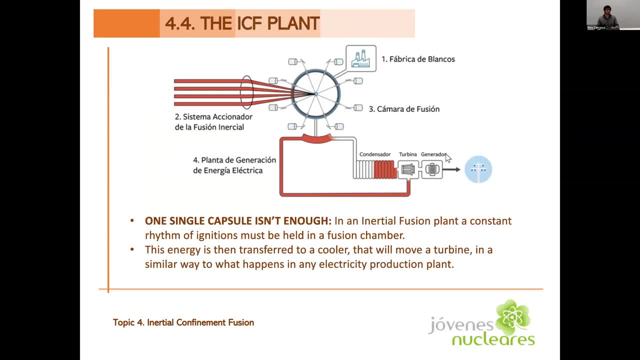 whereas in the, in the central ignition, we only have one laser. so we we can't have this adaptability. no, But it is also more difficult to apply in a plant, because this is more difficult to manufacture. And to finish the presentation, 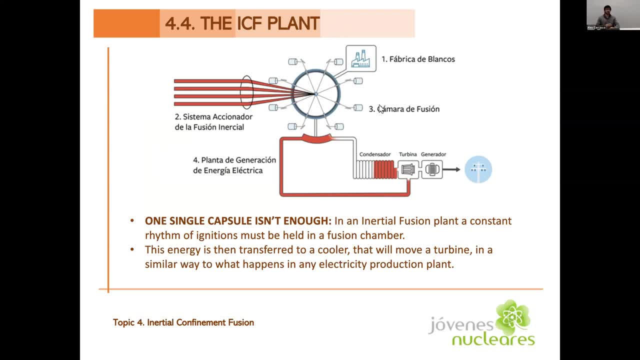 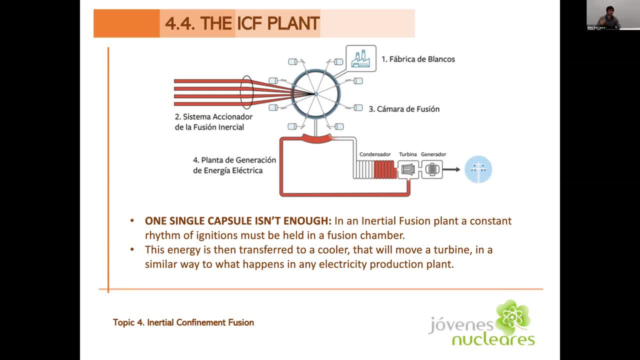 But we need power, We need energy per unit time. So in a, in an ICF plant, in order to produce electricity, we would need to have a, a flow of capsules that would ignite and that would transfer their energy to a coolant. 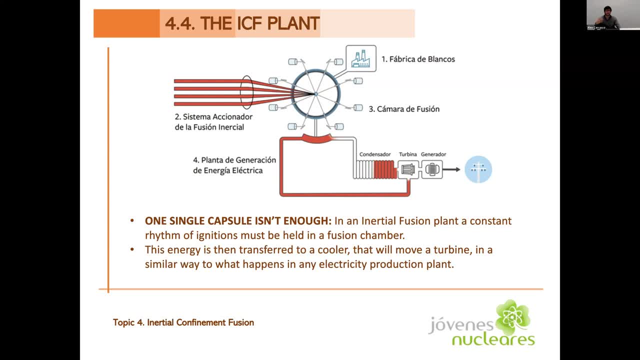 And this coolant would move a, a turb, a turbine, in the same way as a, as a normal power plant, as as current nuclear power plants or in fact any kind of power plant. a coal power plant also works in this way. 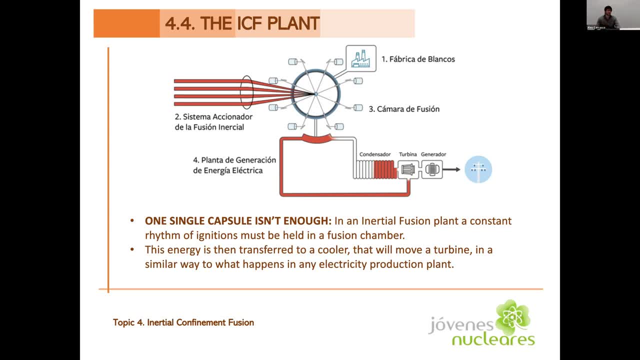 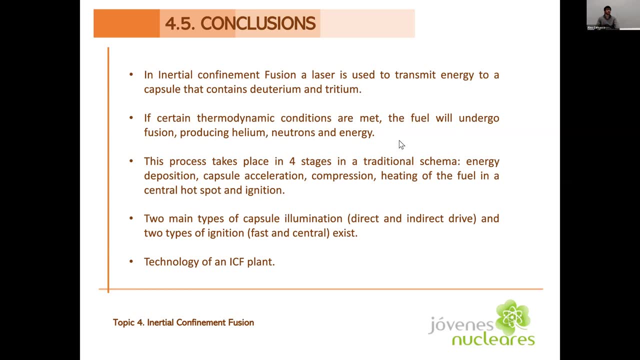 by moving a coolant and producing a certain amount of energy per unit, per unit time. So, as a conclusion to the, to the presentation in inertial confinement. in inertial confinement fusion, a laser is used to transmit energy to a capsule. 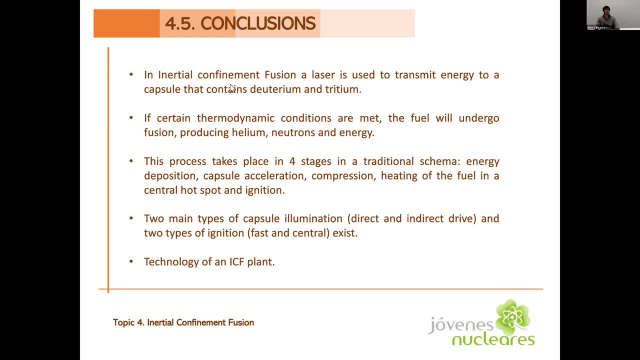 that contains deuterium and tritium. If certain thermodynamic conditions are met, the fuel will undergo fusion, producing helium, newtons and energy. This process takes place in four stages in the traditional schema Energy deposition, capsule acceleration. 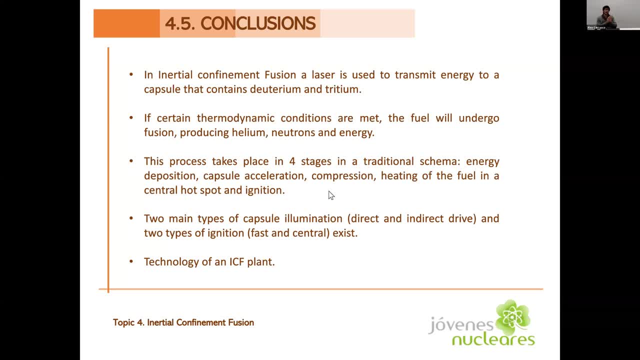 compression, heating of the fuel in a central hotspot and the ignition of the fuel. Two main types of capsule illumination exist: direct and indirect drive. so when the laser shines directly on the capsule and the laser shines on the cylinder, that then produces X-rays. 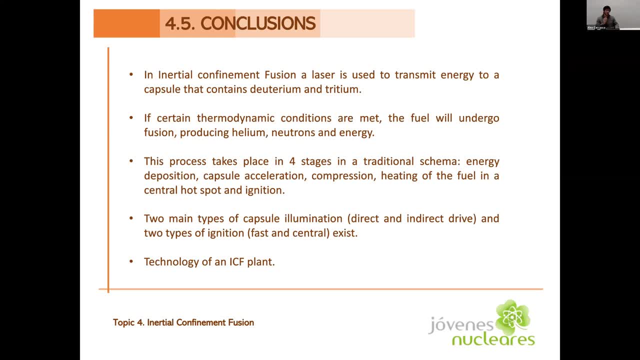 and two types of ignition: fast when we have a spark, and central when the laser is the one that compresses the, the capsule. And we have also reviewed the technology of an ICF plant. So thank you very much for watching. 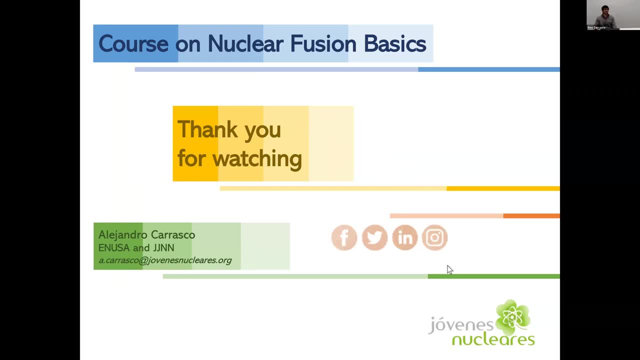 and this is the end of the presentation, and be sure to ask any questions that may arise in the chat, as Paco is telling us. Thank you,